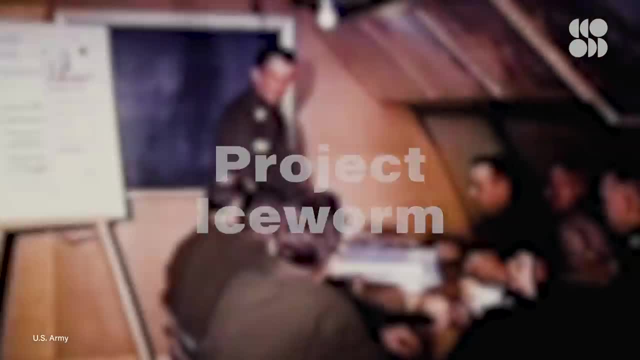 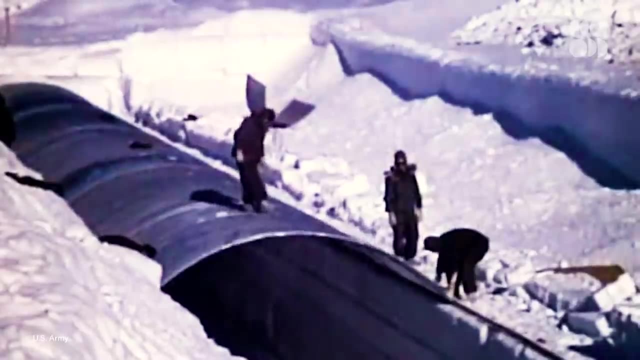 to hide hundreds of nuclear missiles under the ice of northwestern Greenland. Their cover story, Project Iceworm, was just a polar science station named Camp Century. The base had 21 tunnels, a movie theater, hot showers, a chapel, chemistry labs. 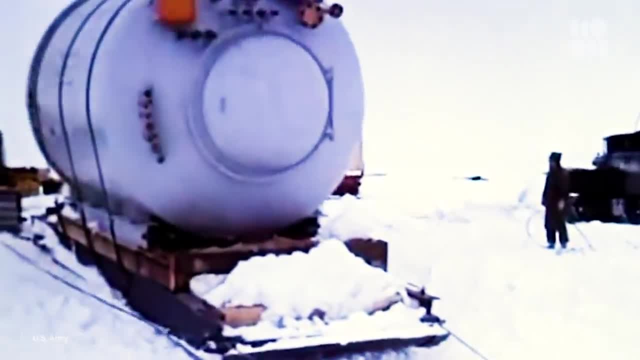 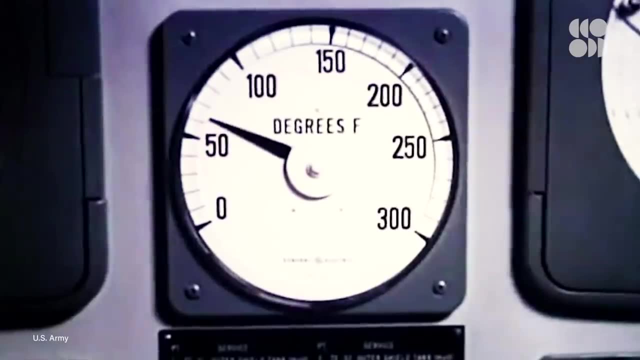 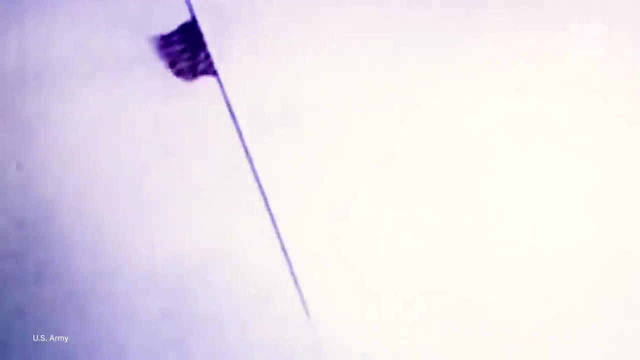 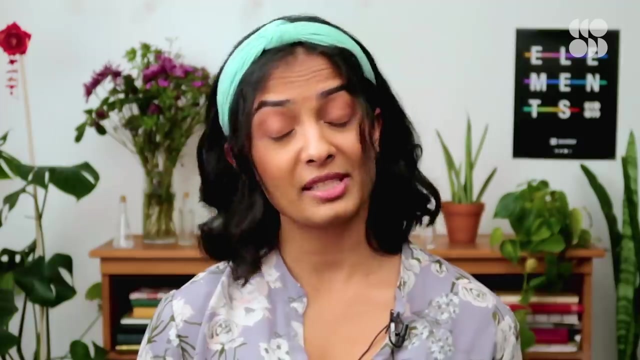 enough room for 200 residents and the world's first port of view, And it was a portable nuclear reactor. Project Iceworm and Camp Century were eventually abandoned due to a heady mix of political disagreement and unstable ice conditions, But since Camp Century was, after all, a polar science station, 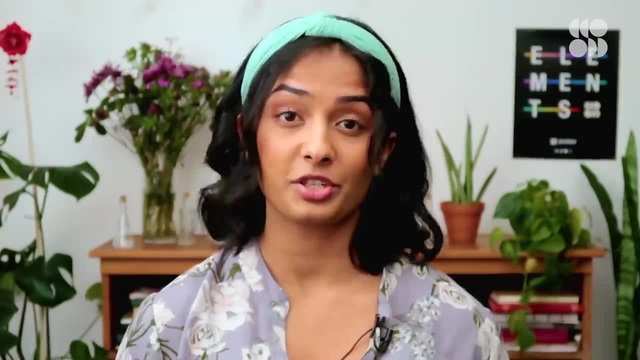 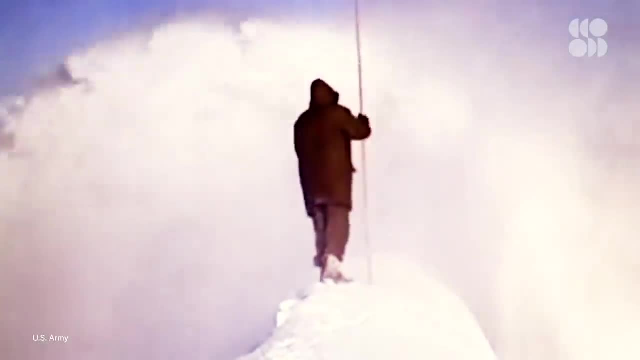 researchers had already done some important work before the whole operation shut down. Although they may not have really done much, They didn't realize it at the time. In 1966, the team dug nearly 1,400 meters down into the ice sheet. 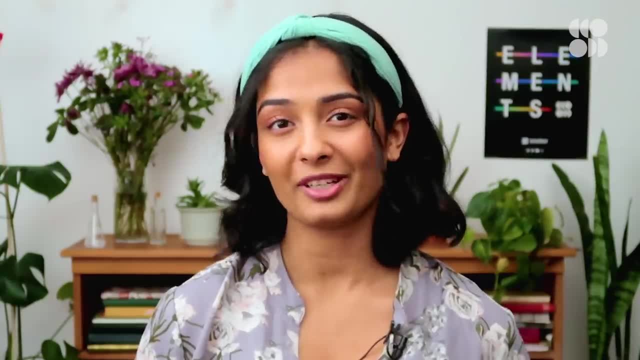 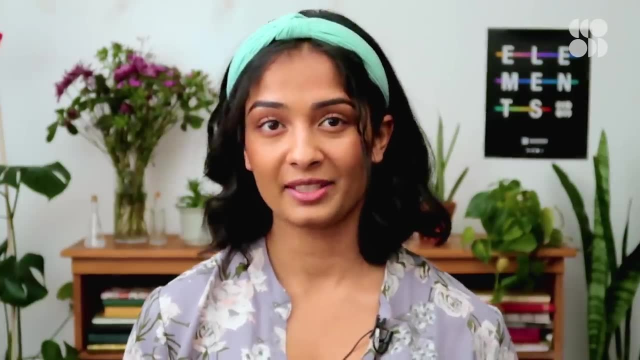 When they finally hit dirt, they took a few cookie jars worth of samples before stopping. Those samples were labeled, preserved in a freezer and subsequently forgotten. Fast forward half a century later when, after their accidental rediscovery, scientists began investigating them for the first time. 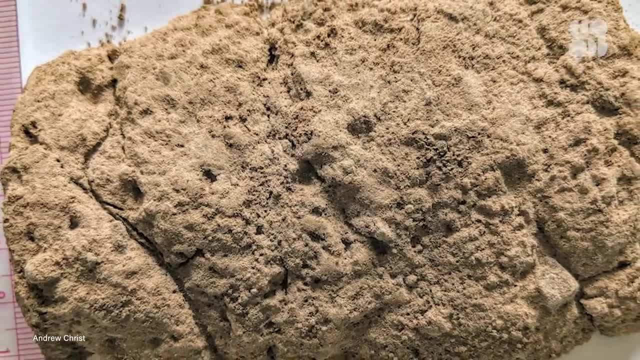 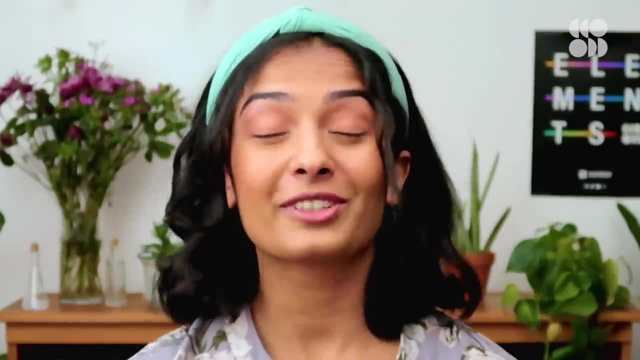 And what they found was stunning. Not only did the samples contain sand and rock, but they also contained the fossilized remains of plant material. Let me emphasize that again, These are perfectly preserved plants. Unlike bones or teeth, soft plant tissues are usually destroyed before they become fossilized. 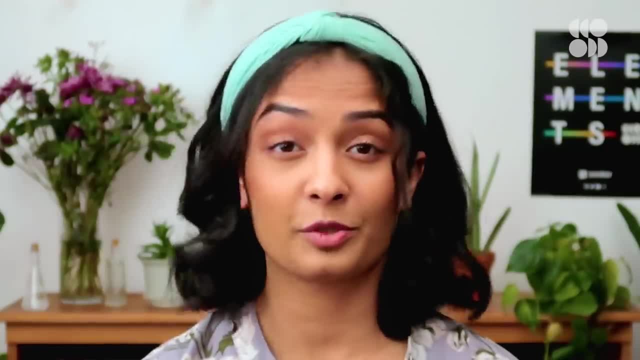 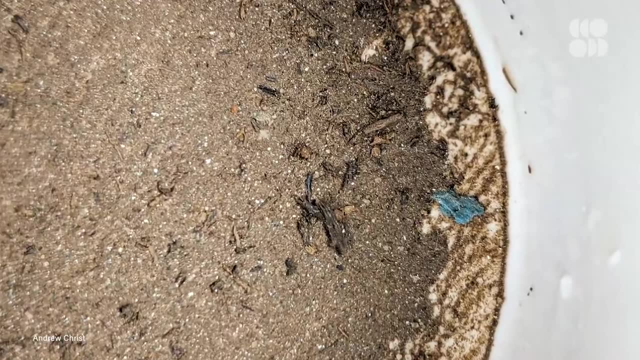 You need really specific conditions and a little bit of luck to preserve them. Past studies have suggested that Greenland was free of ice more than a million years ago, But these Camp Century samples contain perfectly preserved fossilized plants, Which throws that entire timeline into question. 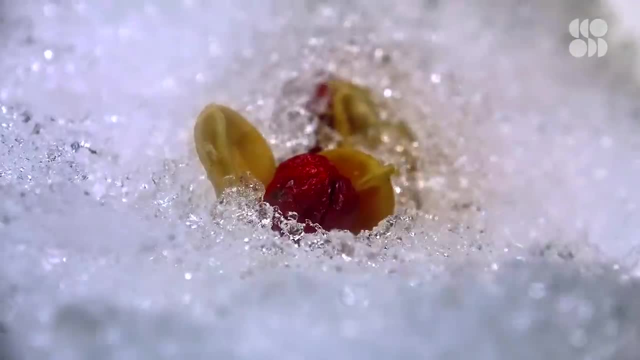 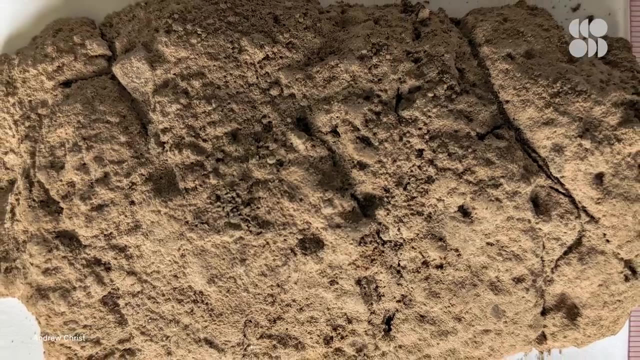 Ice sheets tend to destroy what's in their path And since plant tissue is especially delicate, this means Greenland may have been ice-free much more recently than we previously thought. To help figure out this timeline, the team first looked at an oxygen isotope within the pores of the sediment.